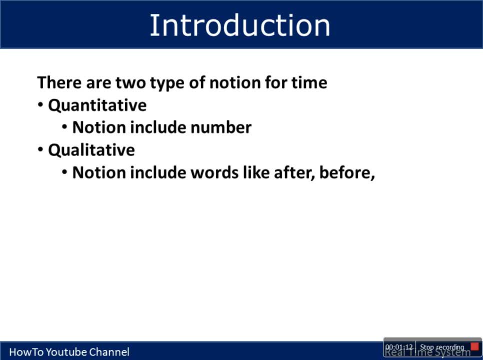 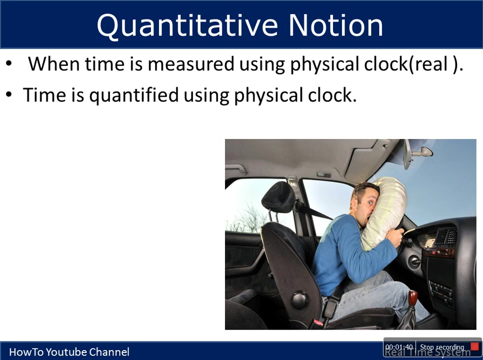 so this is quantitative and second one is qualitative. so here time is represented with the help of words, like before, after like, if a query is given to a system, that system will produce output after that query is processed. so here this notion will be using words, whereas quantitative will be using numeric. so in quantitative notion, how? 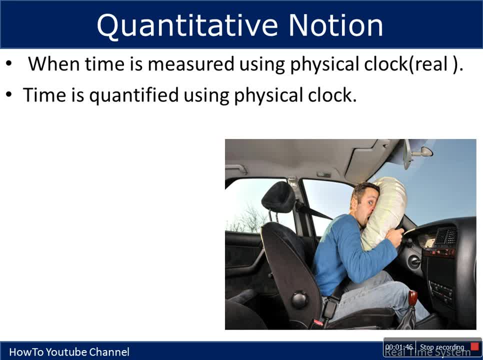 this numeric time can be achieved, so there will be a physical clock and time is quantified with the 것 like that clock. let's say, for example, now a day, in every car we are getting airbags, so whenever a accident occurred, that air bag has to be opened within a minus second. so who is specify that after? 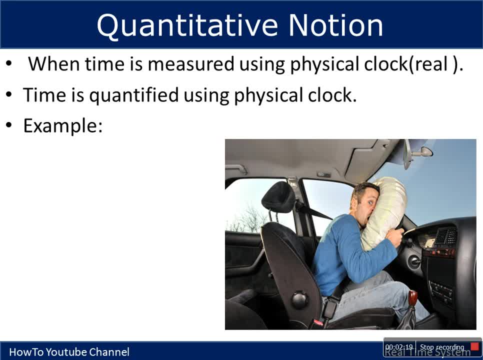 accident after lapsing three micro second, this bag has to be open, so there has to be a physical clock. after lapsing three microseconds, this bag has to be worry about being cornered by a calendar of three second, so there has to be physical clock. so after that accident, after lapsing three micro seconds, this 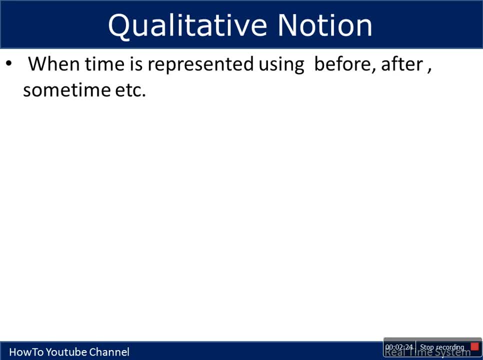 has to be open. so therefore, this watch has to be physical clock and there has to be a time to choose digital clock�� panelists. please, in the comment box, I will explain to each of these examples. and clock and qualitative. we have seen example like query, when a user is giving. 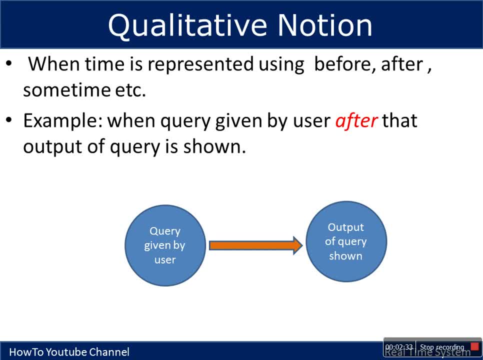 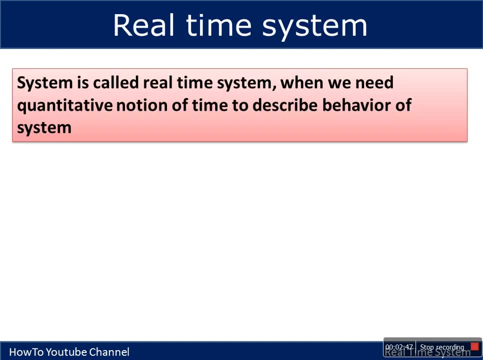 credit to a system, that system has to produce its output once it saved that query. so these were actually specify the sequence of operation. there is no particular numeric number used. now let's see what is real time system. so before going to discuss real-time system, just discuss a system. normally, when we have a 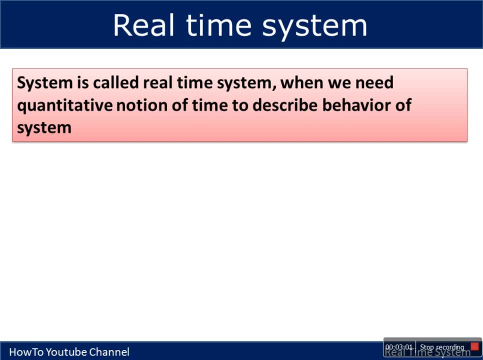 system how we going to identify whether that system is working properly or not. we will use that system and output given by that system. we will compare that output with the actual output. so if both compare, it means that system is working perfectly. but in case of real-time system, first thing you need to remember: 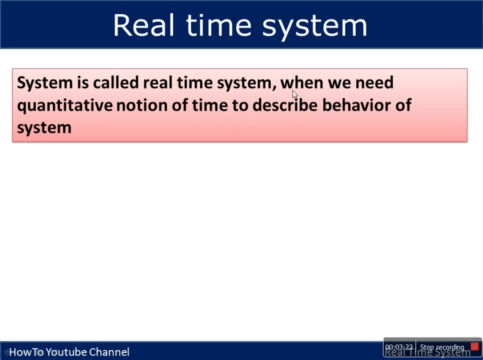 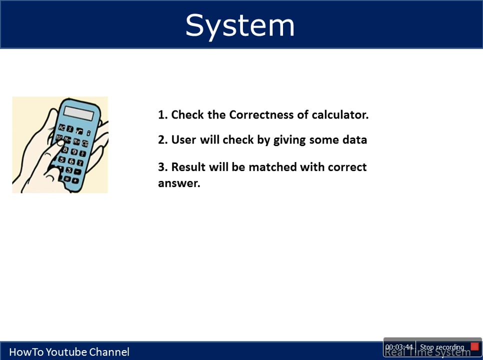 time the system. actually, in this system, time is used to describe behavior of system, and which notion of time a time is used- quantitative motion? okay, so in real-time system, quantitative notion of time is used to describe behavior of a system. how, let's take this example. let's say we are having a calculator and we 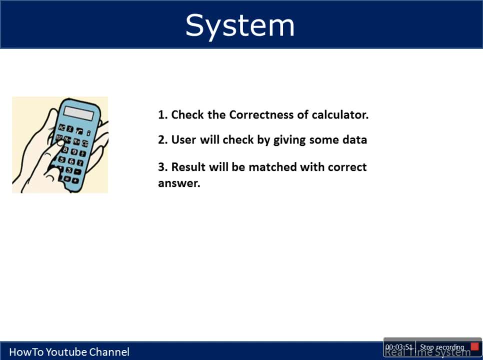 want to see whether this calculator is functioning properly or not. so what we will do, we will give some input to calculator. this calculator will give us some output and we will compare that output with the actual output. so we know that 2 plus 2 is equal to 4 and 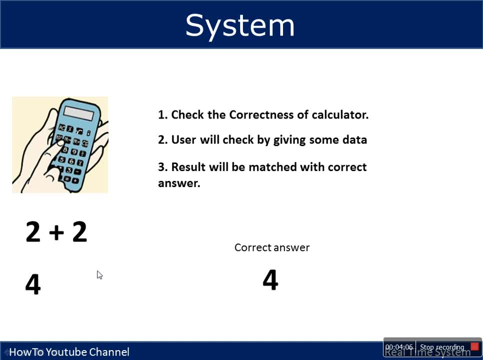 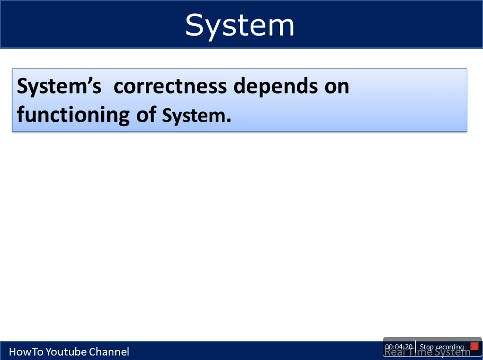 calculator also giving this output. both are same same way. we will do some other operation as well. so if all output match, we can conclude that our calculator is working properly. similarly, a system's correctness depends on functioning of system only. but in real-time system a system is considered correct if that system is performing. 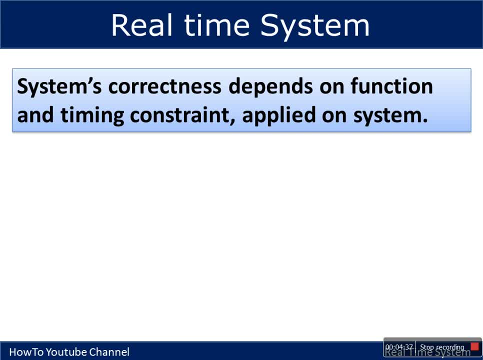 correctly with some time can straight. so when this correctness criteria include functioning plus timing constraint, those system are actually known as real-time system, bag deployment system. that system has to be active within one or two millisecond so there will be a time constraint. so if that system is working after that time, 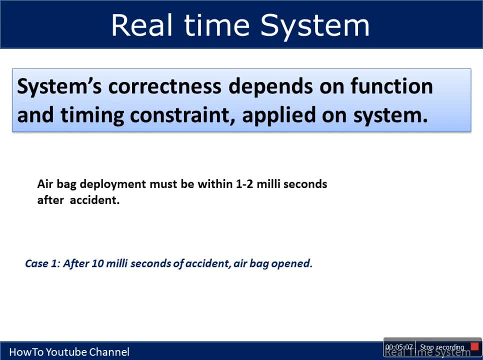 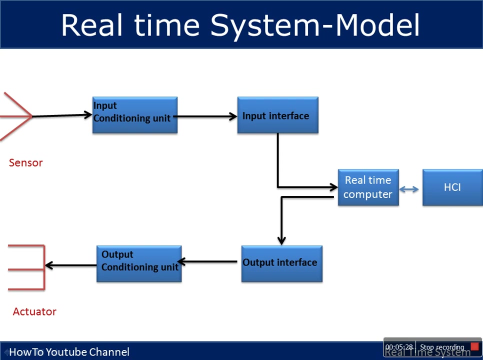 constraint, that system will be considered fail. so after 10 millisecond of accident airbag open, in that case this system will be considered fail. so here now a new criteria is defined for the correctness of system: time plus functioning. this is the architecture of real time system. we are having sensor. 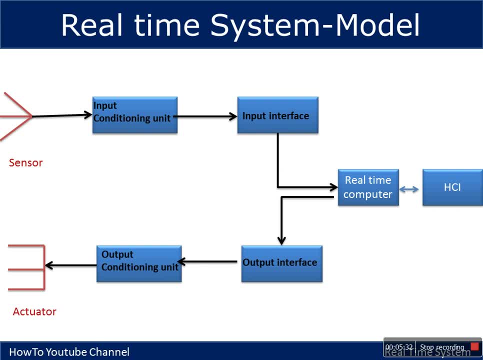 this sensor will sense and provide input to input conditioning unit. now, this signal provided by sensors or data provided by sensor are very low. their voltage level is very low- so this is the architecture of real time system- and very low. so this input conditioning unit, it will amplify those signals and 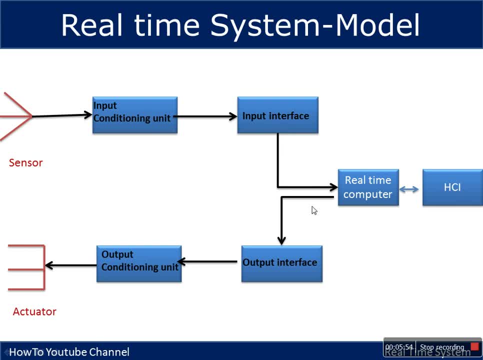 provide it to input interface and through this interface real time computer is connected. so here all the processing is going on and this one is connected with SCI to which a human can interact. so similar we are having for output interface. output interface will provide signal to output unit. this unit will convert the signal according to actuator and then these: 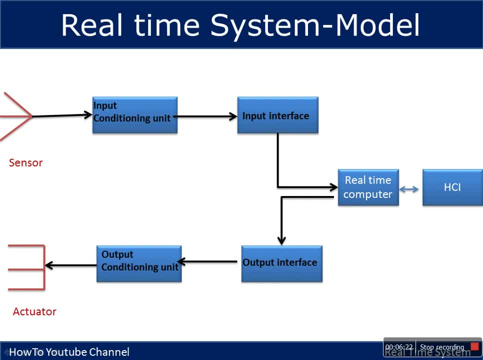 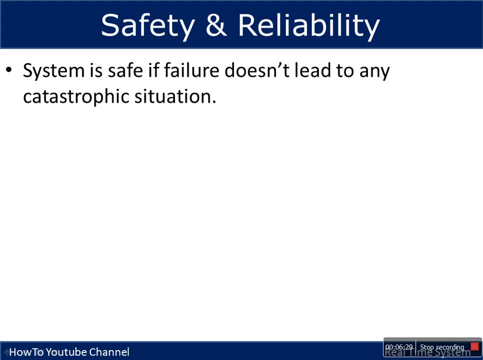 actuator actually will perform actual work. now let's discuss these two features: safety and reliability. so when a systems is safe and when the system is not safe. so if a system is safe and if failure doesn't lead to any catastrophic situation, this one has to be followed in system. and the reliability. what is reliability? reliability, ability to perform. 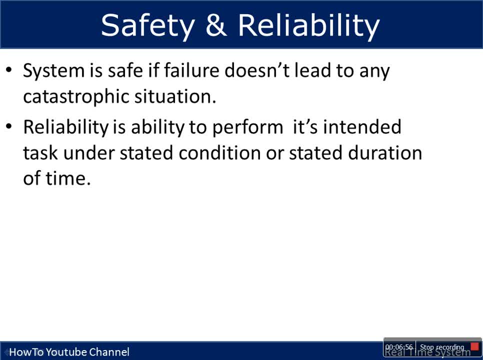 its intended task under stated condition or stated duration, like if you are buying a system and that system supposed to be functioning for five years. so if that system is working perfectly for five years it can be considered a reliability. so reliability- how long that system is working perfectly- in case of failure as well. so in traditional system, safety and reliability are. 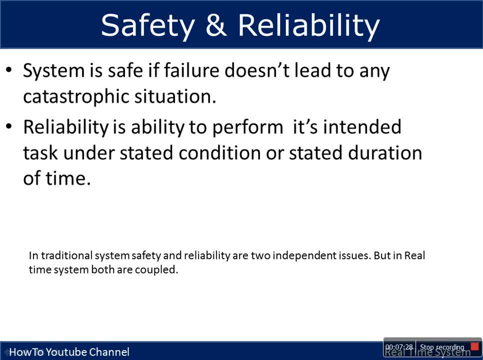 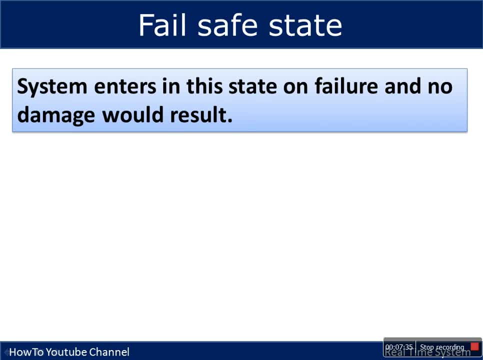 two independent issues, but in real-time system the both are coupled. how so feel safe state? so whenever a system is failed, at that time, in order to avoid all damage, there will be a state, and so whenever there is a failure, system will enter into that state. that state is known as failsafe state now. 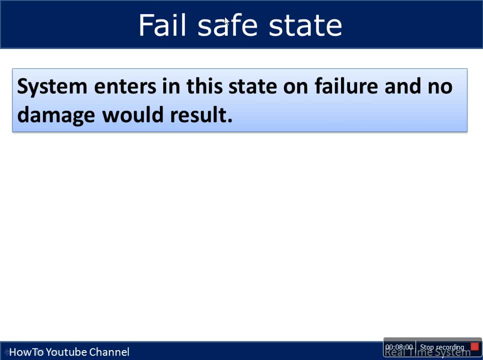 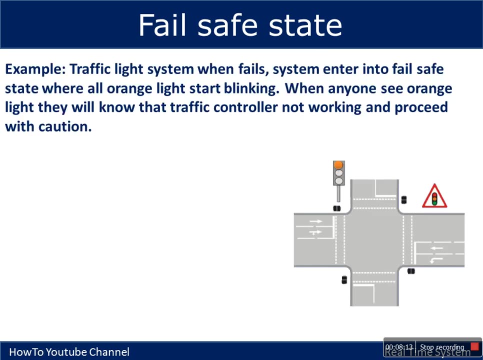 you need to remember this: that for all real-time system we don't have failsafe state. for some real-time system there will be this state, but for others there won't be any failsafe state, like we are having a example of traffic light system. so whenever this traffic light system 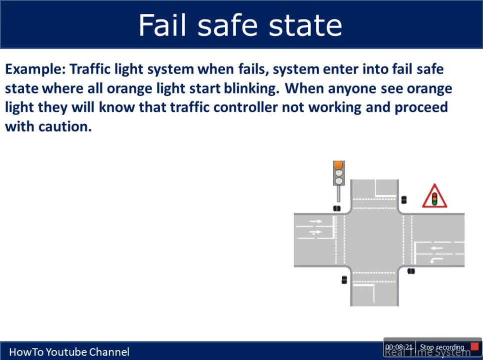 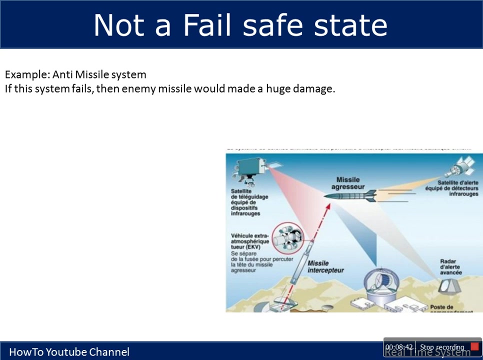 fails system will enter into failsafe state, how it will start blinking orange light. so when anyone will see that orange light, that person would know a traffic controller not working. so proceed with caution. so there is a failsafe state, ok, and anxiety. but in case of anti missile system, in this case, if this system fail, that 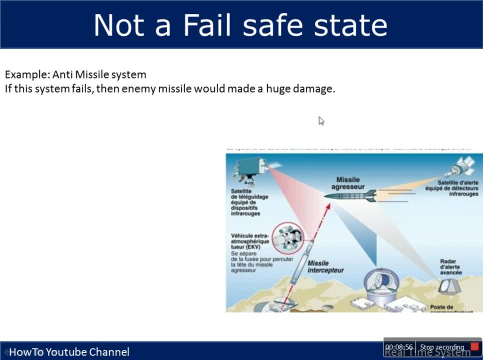 would result in a catastrophe that would make a huge damage. so here many team's vitals system. there is no failsafe state once a missile is long and if there is any problem 보고 with missile interceptor or any kind of problem occurred, this will be missed and 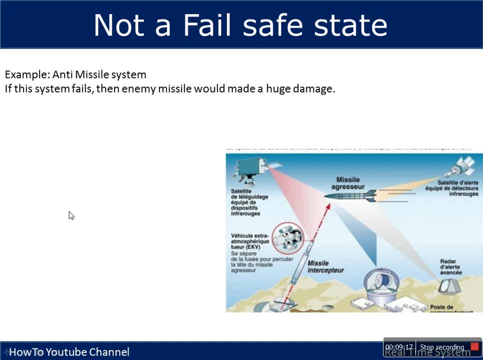 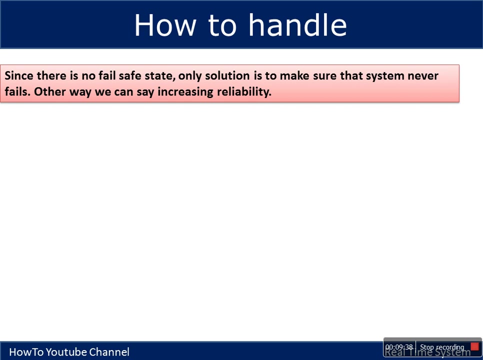 it would result in a huge damage. so there is no failsafe state. so these type of systems, known as safety critical system- system for which there is no failsafe state, exists, those system is known as safety critical system. now the question is that, if there is no failsafe state, how to make sure that? 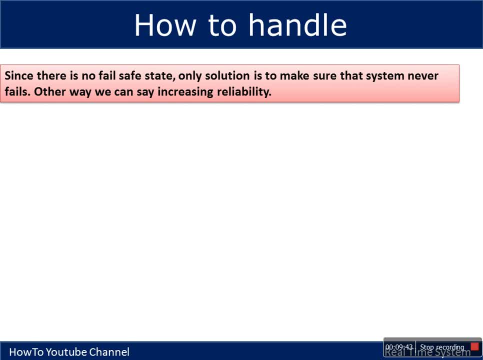 that system would not make any damage. so the only solution is that we need to increase reliability of those system. so how can we increase this reliability? when we are having a system, there are chances that any component of that system stop functioning or the program stored in that system. 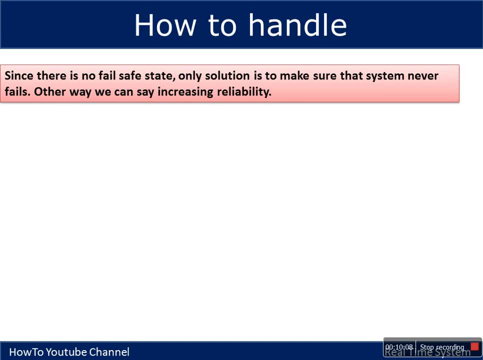 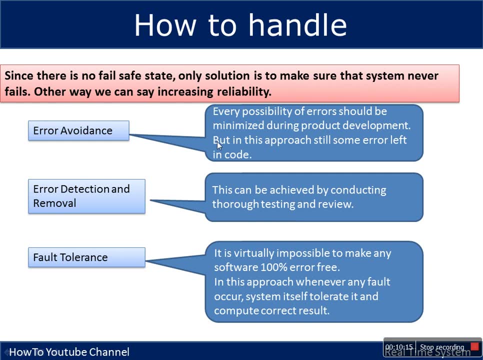 stop functioning, there can be a bug. so there are multiple ways. first is error avoidance. so it states that every possibility of error should be minimized during product development. but it cannot be achieved, like whenever a system is in development, some errors are left. second one is error detection and 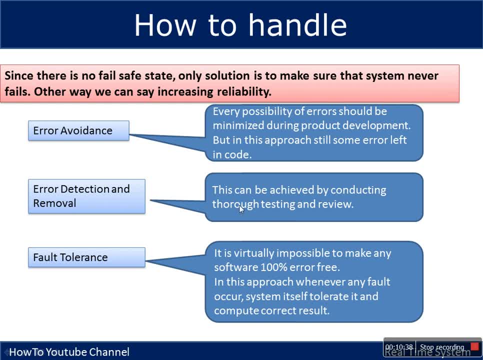 removal. so this can be achieved, like a system can be tested again and again and then, on the basis of test result, that system can be updated. and third one: fault tolerance. so the thing is that we cannot create a system hundred percent error free. there will be error, so if that system is capable of handling its 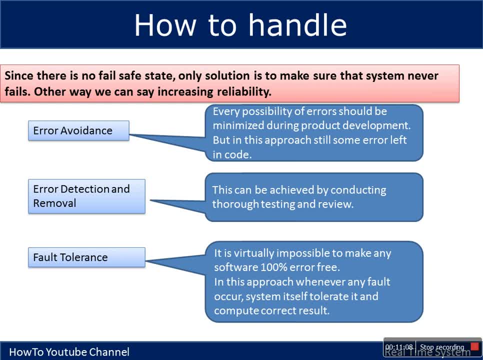 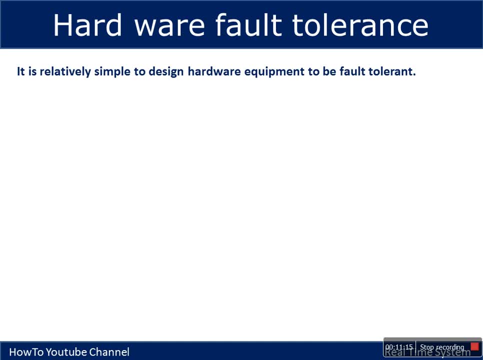 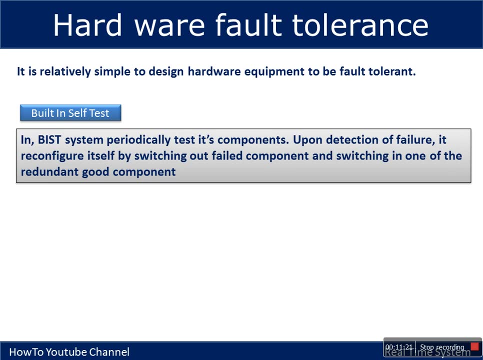 error on its own. so in that case reliability can be achieved. so we are having two type of fault tolerance, for one for hardware, another for software. so for hardware fault tolerance, first approach is that built-in self-test, so this component will test every other component in a system. so on the 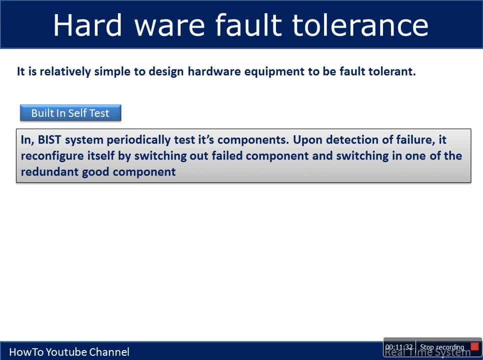 detection of a failure. whenever it will find there is a one component is not working perfectly, it will switch out that component and it will switch in another good component. so for that case, for every component, there will be a redundant copy. so whenever one component stop working, another component will be used and the 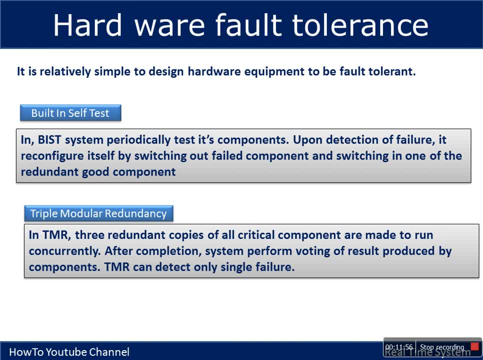 second approach, triple modular redundancy. so it it stated that for every component, three redundant copies of those will be used to run concurrently. now let's say in component, so in a system, that system is performing some tasks and in that system, for every critical component, they are three. 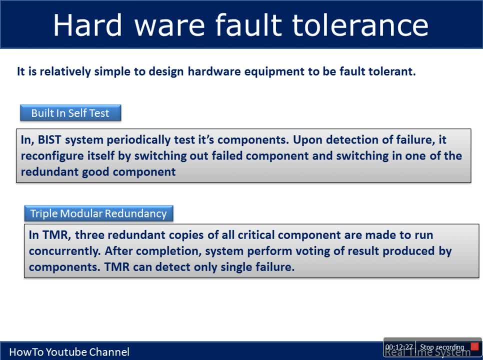 copies. so whenever that task is completed, at the end voting processes started. so it will be seen that all the components- this is the order systems, will get COPIED and in addition to this, for every component three copies will be used. so that system is performing some tasks and in that system, for every critical component there, three copies. so whenever that task is completed, at the end voting process is. 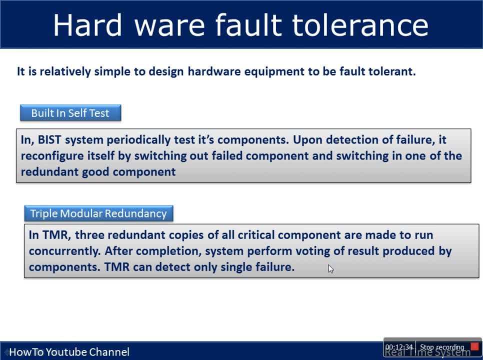 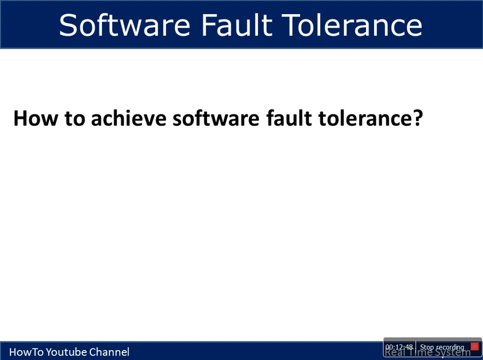 started. so it will be seen that, out of three, if two copy giving one output and one copy giving another output, so it will be in the favor of those two copy. now there is a question like how to achieve software fault tolerance. can we use same techniques which are used in hardware fault tolerance? so the question: 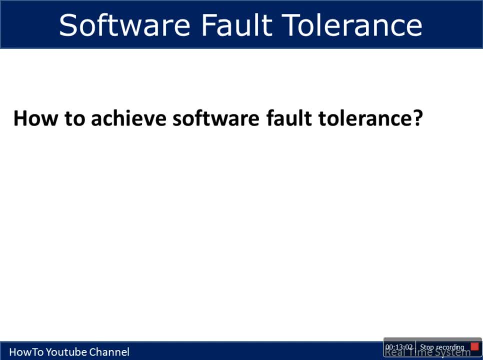 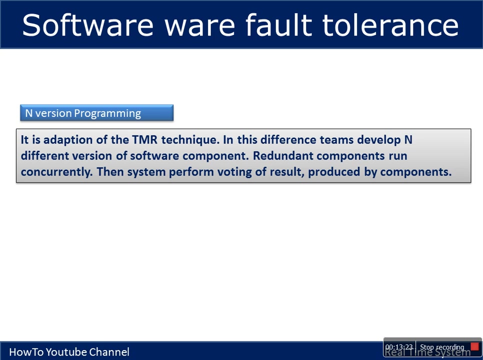 is so, answer is that you cannot use same technique. so so for software fault tolerance, there are number of techniques. we are going to see only two. so first one is n version programming. so in n version programming, for every module, different, different team will work on that module and they will provide. 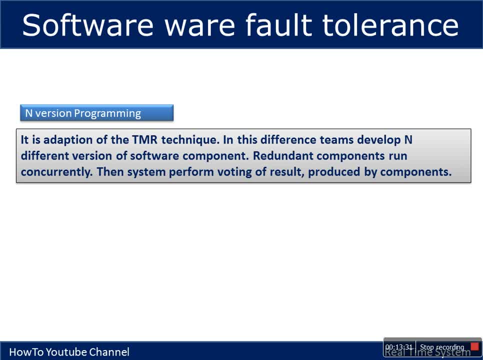 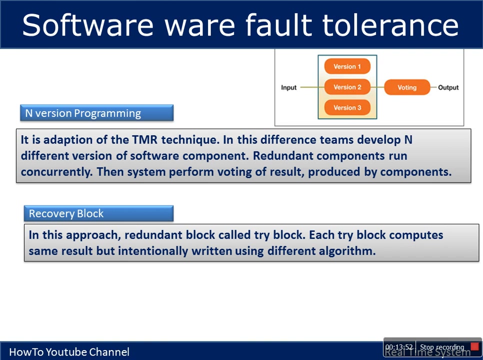 different modules for same task and whenever a task has to be completed, both all those that module will be used and at the end voting of result will decide correctness of the system. so this is n version programming and second one recovery block. so in recovery block for every module there will be a redundant block. 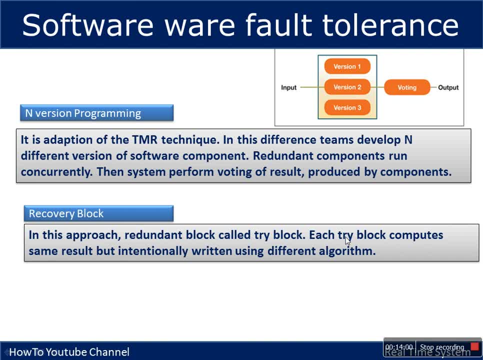 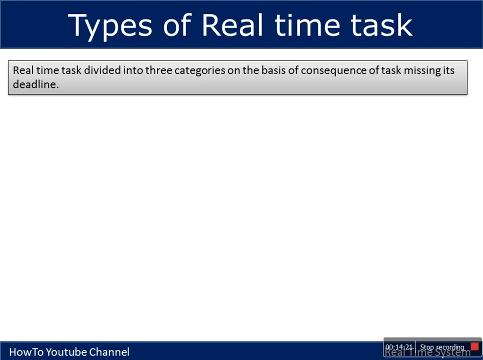 and that is also known as try block, and every try block compute same result but intentionally return using different algorithm. so intentionally, during development every team will use different algorithm to calculate same result. so this approach is recovery block. now let's have a look on types of real-time system, so how these categories are actually made. 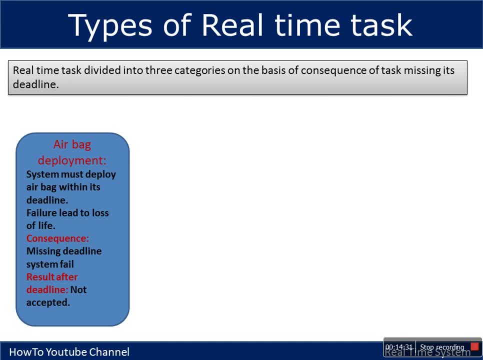 so these category first see the example of this particular real-time system: airbag deployment. so we know that if this airbag deployment system missed its deadline, like if this system doesn't work in a particular time period, it will be considered failed. so what are the consequences? missing deadline system will fail and after those, 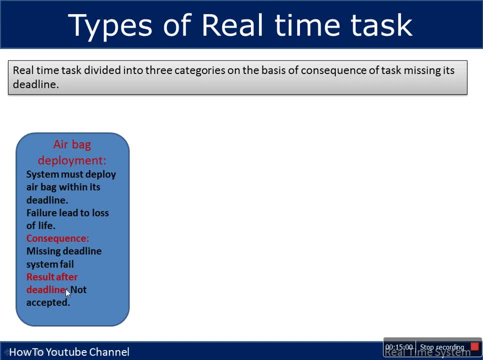 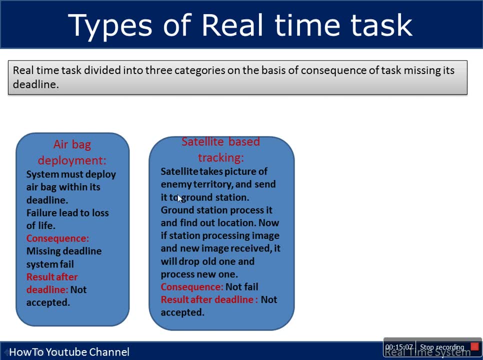 time consideration. if that system is performing, there is no use, so not accepted. now let's see the another example: satellite based tracking. so in this example satellite will take picture of enemy territory and send it to ground station. now let's say the ground station is busy in processing received images. 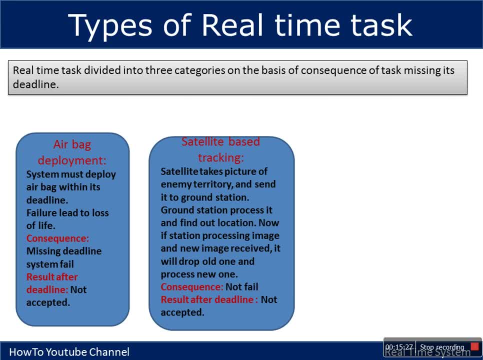 and meanwhile a new images are received from the satellite and that system actually missed to process those images. and so in that case, what will happen? that system will not be considered failed, but the result after deadline, those result will not accept it, like if a satellite has sent some images at a particular time and that ground station not able to. 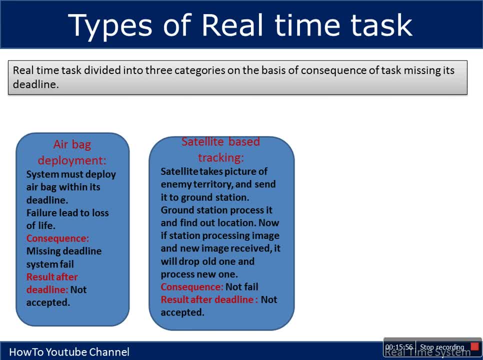 process those image. so after some time that satellite will again send the images. so what this ground station will do? that ground station will discard the previous images and it will accept the new one. so our system will not be considered as failed. but whatever result it's getting after deadline, those 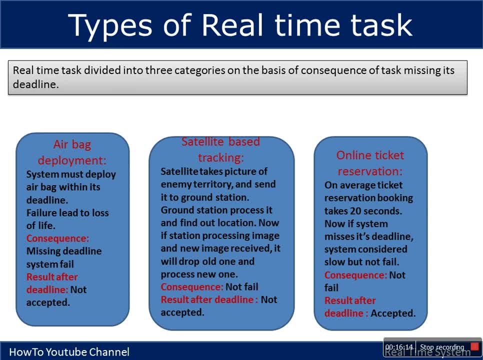 result: not accept it. and the third one, online ticket reservation system. so in this system we can say that when we try to any seat it will take 20 to 30 second. now if that system is taking more time, let's say that system actually took 40 second or 50 second and after 50. 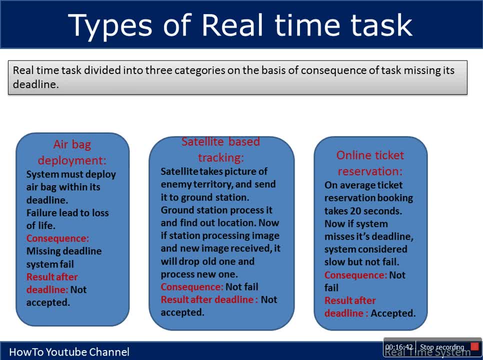 second, that system actually booked seat successfully. so here there is no role of deadline. here. if the deadline is missed, system will not consider it paid, and after that deadline as well, if the reservation is successful after 30 seconds. so it actually missed this deadline. after that deadline as well, result excepted. so we are having three. 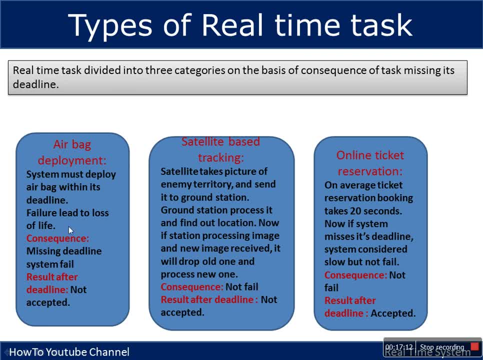 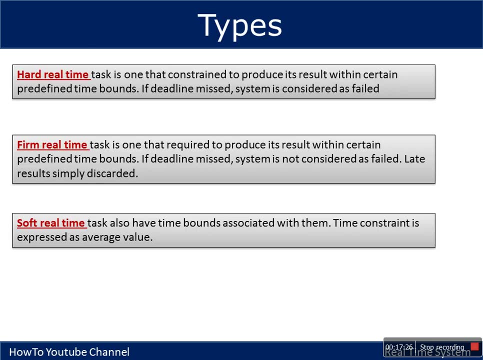 types of real-time system. so, and these gatek? we actually decided on the basis of this one whether the results are accepted after deadline, or 재미's, or not, and what are the consequences. so, on the basis of these three, we are having three different type of real time system: hard real time system, firm real time system and soft real time system.